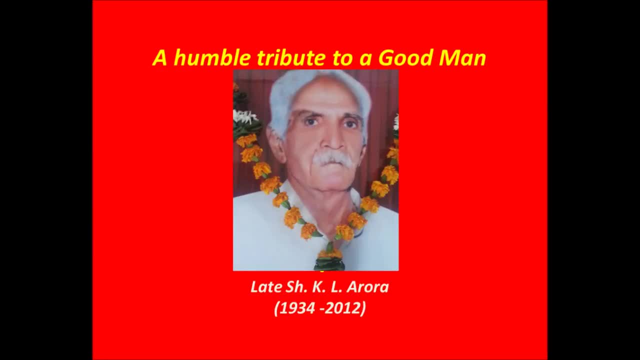 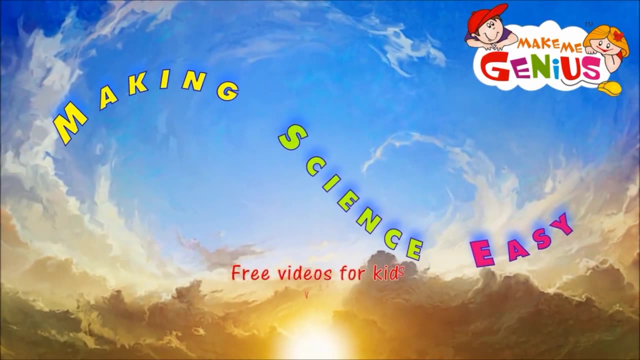 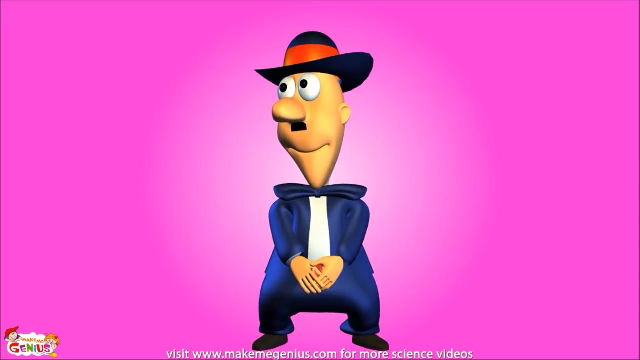 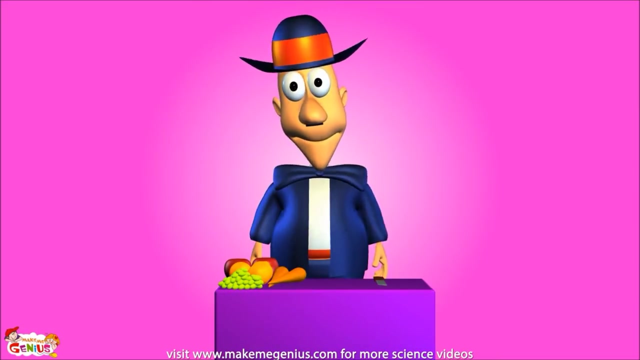 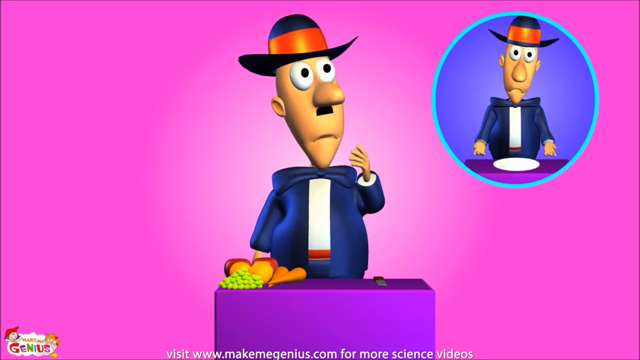 Wow, you're a good dancer. It seems like you really love fruits. But did you know that in the future we may not have any fruits? In fact, we may not have any food at all? Yes, you're right: No fruits, no food. Now one question: Do you know where all fruits and food? 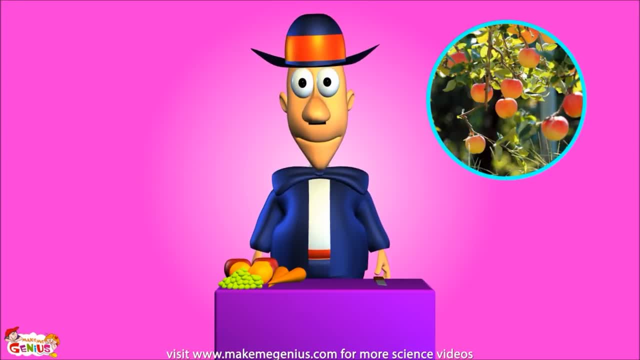 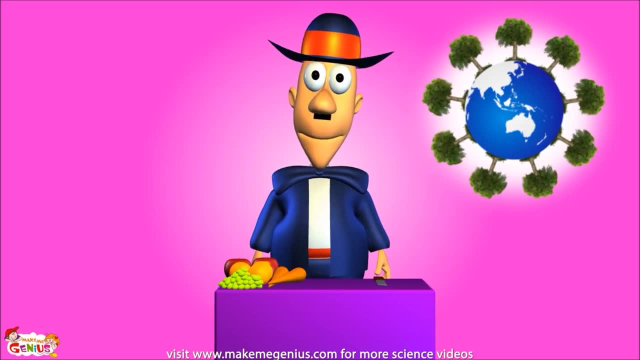 come from? You're right, All food comes from plants. But do you know where plants grow? You're right, Plants grow on our planet Earth, on the Earth's crust, But did you know we're not able to grow plants everywhere on the Earth's surface? The area where we can grow fruit is 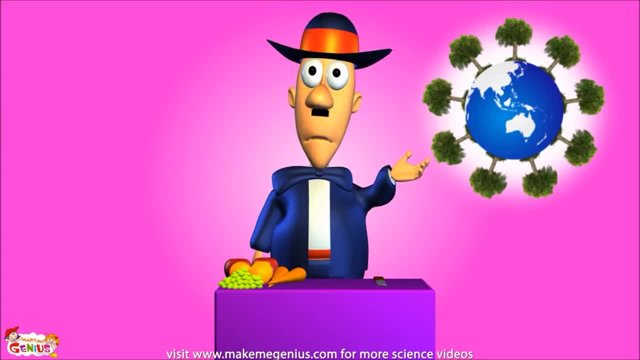 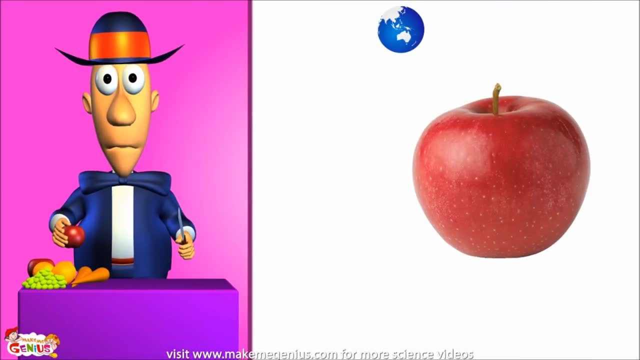 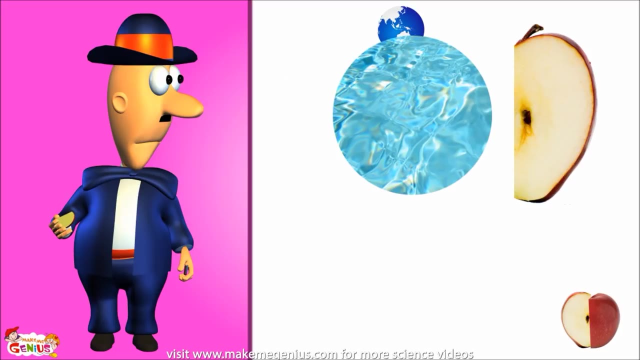 very, very limited. Okay, you don't believe me? Let's use that apple and knife as an example. Think of the apple as the planet Earth. Now can you tell me how much of the Earth is covered with water? Yes, you're right. If we cut the Earth apple in four parts, three of those parts would 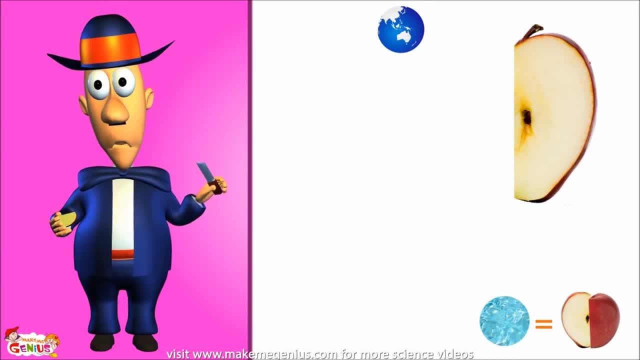 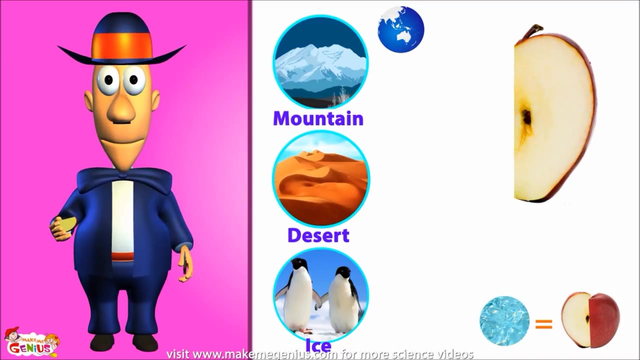 be water, So we can't grow any food plants there. So only one-fourth of the Earth there is land, But again, we can't use all the remaining land not covered by water to grow fruit. Do you know why You're right? On half of this available land we have mountains. 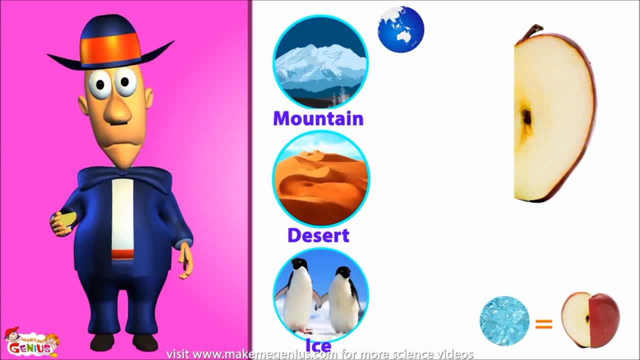 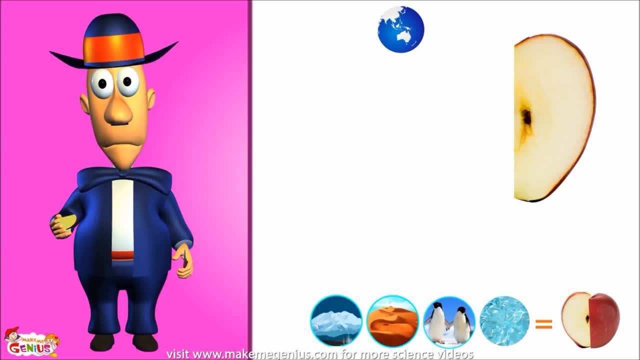 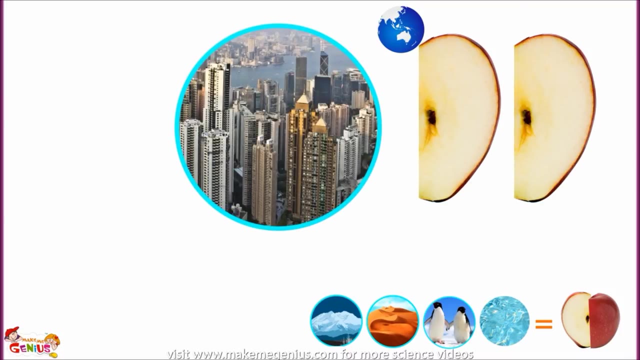 deserts and ice, So we can't grow any plants for food there. So let's cut this piece of apple into two parts. Now we're only left with an eighth part of an apple. Hmm, one-eighth part of the Earth Now. on this part, we have cities, buildings, roads and a place to grow plants for food. 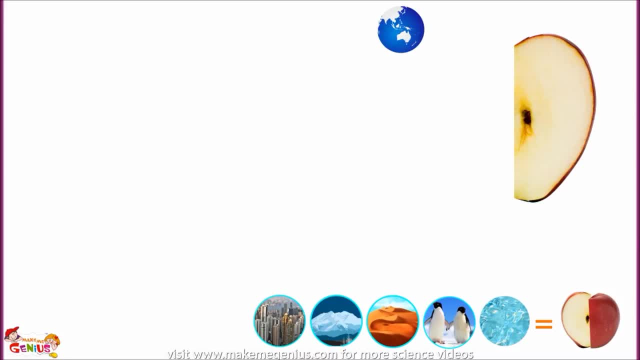 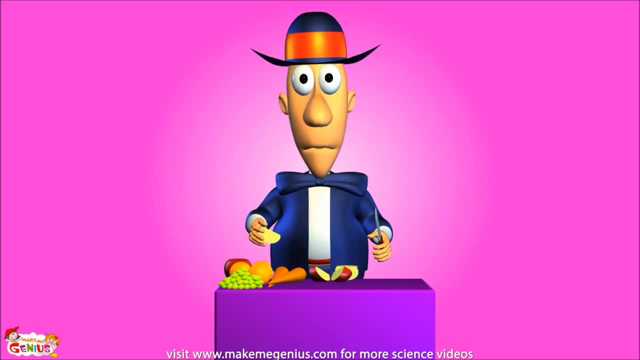 Did you know that only one-fourth of this part is available for growing plants? Oh, you look worried. So this is the only piece of land where we can grow our food. But did you know we can only grow food on the topsoil of the land? Please peel this piece. So this little piece of skin is the only. 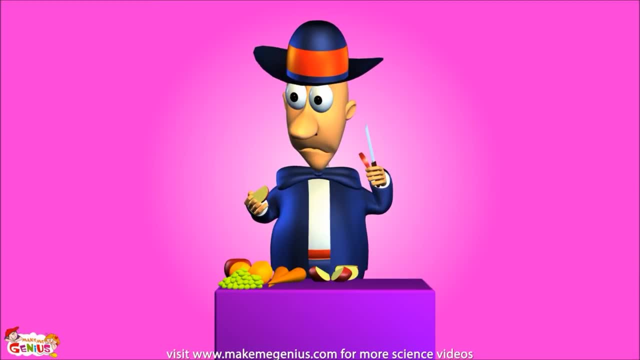 place where we can grow food. Oh, you're saying we also have that part available for growing food. Ah, for that you need to understand the soil profile. Only on topsoil can we grow plants. Come with me into the garden and let's understand why only topsoil can be used. 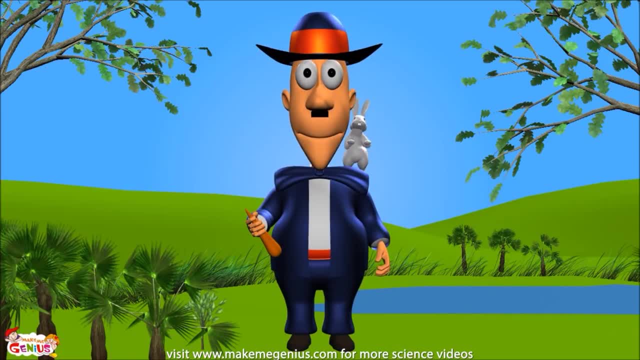 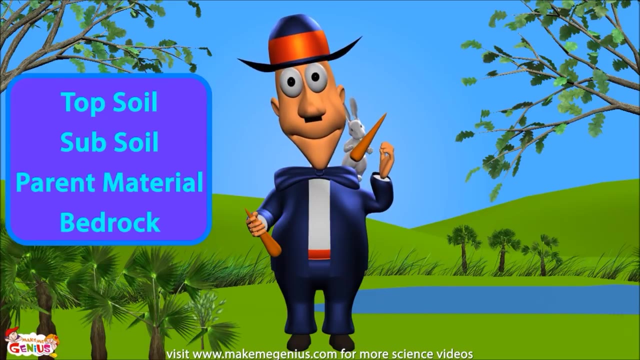 Wow, is that your rabbit? That's why you brought carrots. Oh, he can help us here. Look at the soil in this garden. Our soil has four layers. These layers are topsoil, subsoil, parent material and bedrock. Can you ask your rabbit to dig a hole for us in the soil? 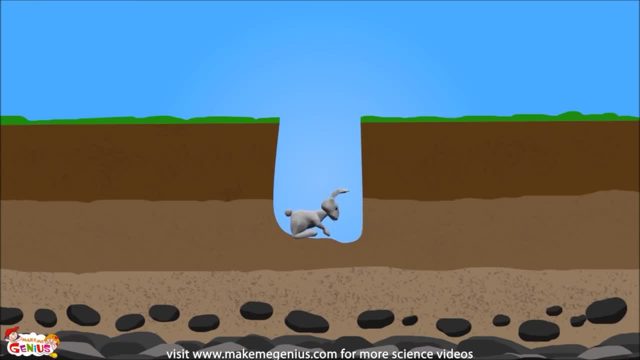 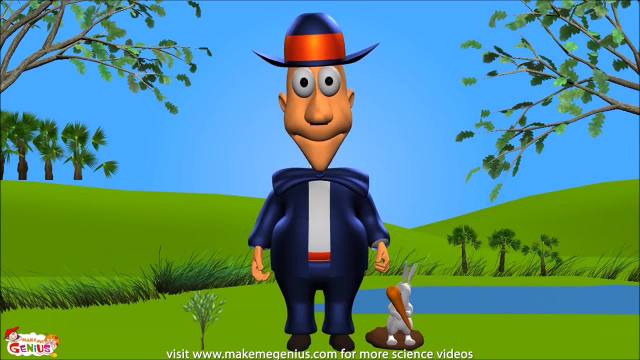 Rabbits make their homes in the soil by digging holes. They can dig really really fast. Great, he is really quick. Oh, I see you're rewarding him by giving him the other carrot. Now let's look at different parts of the soil. The part in which your stick is showing is called 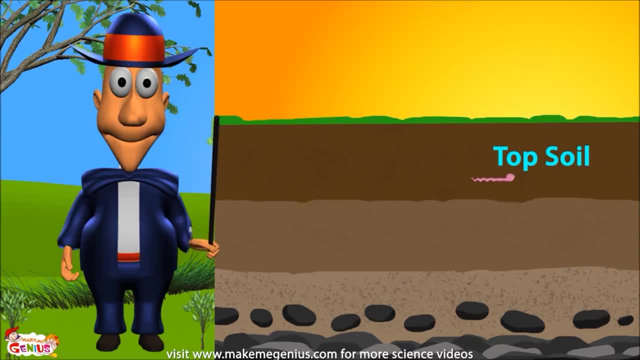 the topsoil Plants and trees grow here. It is very rich in nutrients which are good for plant growth. It also contains lots of worms which are helpful for plants. The upper part is called the humus, which has a lot of dead leaves and dead animals. These dead leaves and animals are slowly. 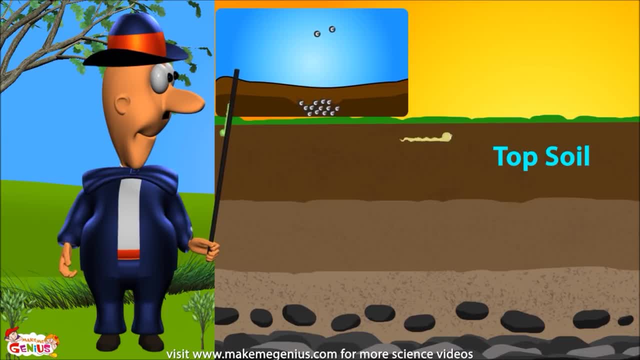 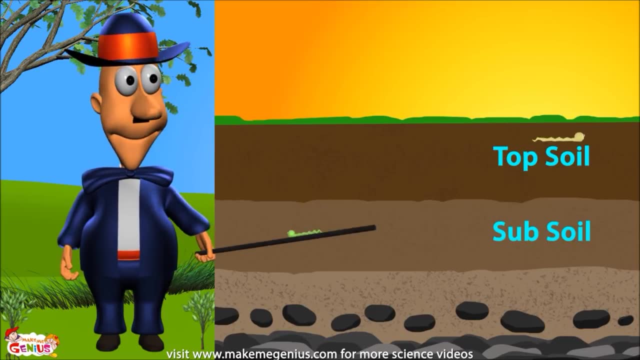 decaying. with the help of soil bacteria, This process helps form organic nutrients which are necessary for plants to grow. This part is called subsoil and has small particles of rock. This part is called parent material. These are the parents' rocks which get broken down slowly and become smaller and 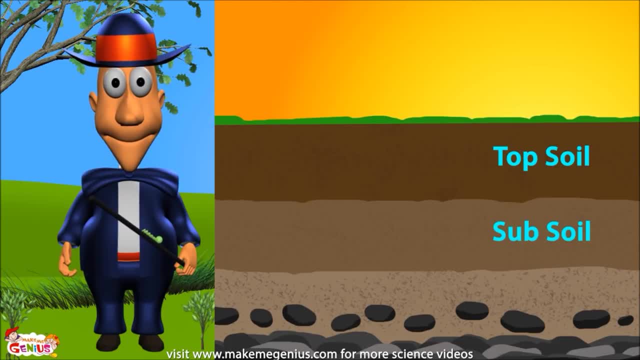 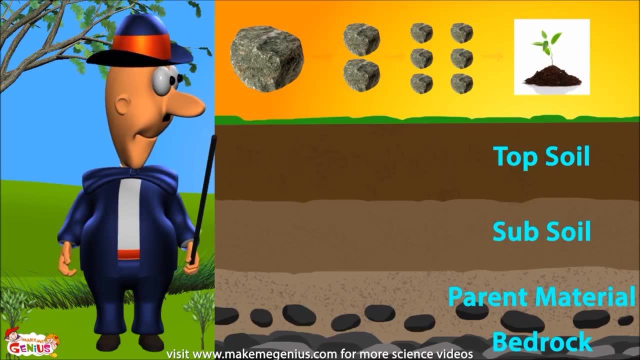 smaller to form the soil. So this is the part in which the parents of topsoil and subsoil live. Aha, these are big rocks. These big rocks are kind of grandparents of the soil. They break down and form the parent material. Then the parents' rocks break down due to the pressure temperature. 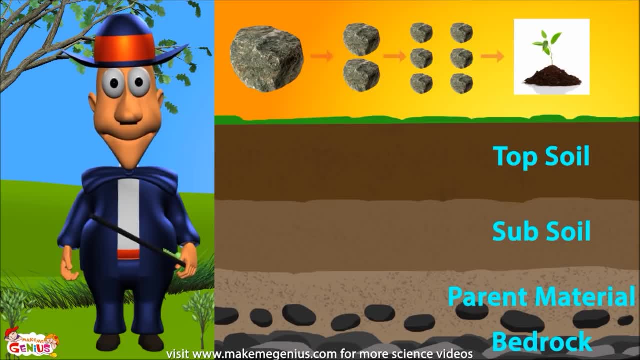 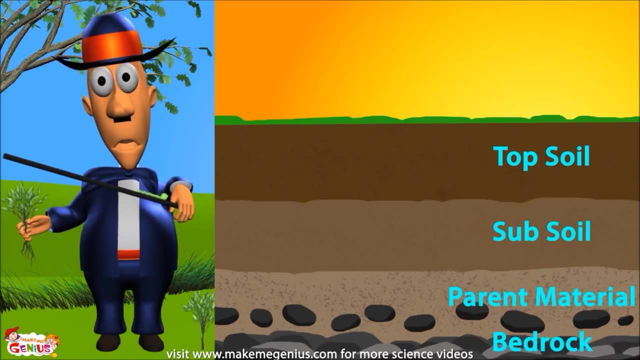 and water. This is how subsoil and topsoil are formed. Please uproot a plant. I want to show you something. Oh look, it's an earthworm. Don't worry, they aren't harmful. Earthworms are a friend of the soil and plants. Okay, now we have. 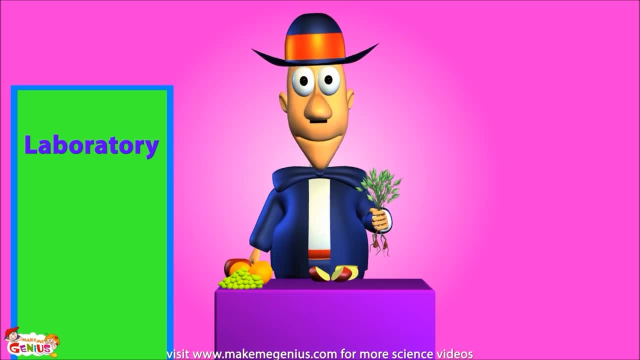 to study in a classroom. So now you know why topsoil is important for us, as it is the only place where we can grow food for ourselves and other animals. See what a small portion of the earth we have for growing plants Food. Did you know that it takes 500 to 1,000 years to get one inch of topsoil? Yes, nature. 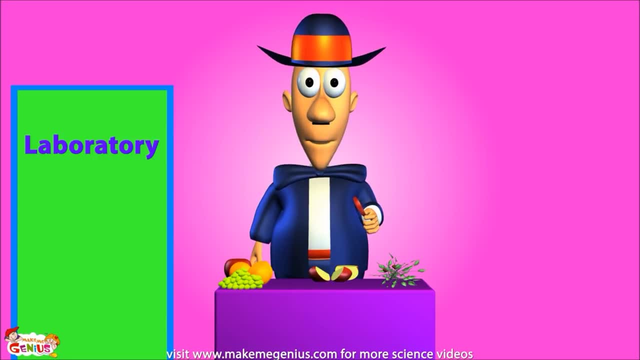 takes many years to make even an inch of topsoil, But did you know that even this tiny part is in danger? Yes, this part is getting smaller and smaller due to soil erosion. Oh, you didn't know about soil erosion. It is about our topsoil getting washed or blown away by water and wind. 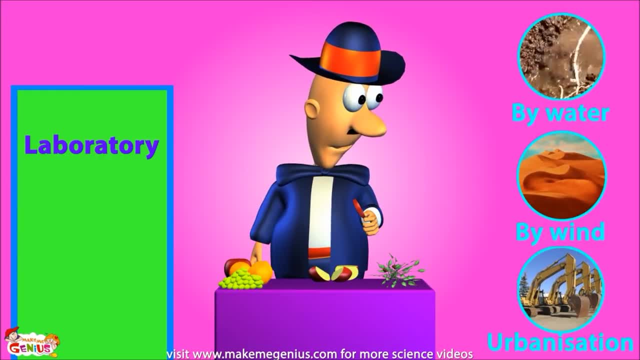 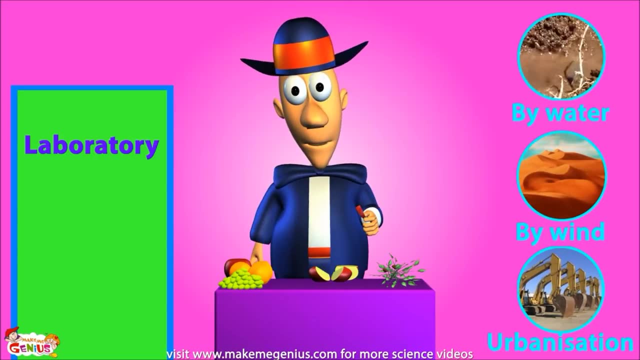 We humans are also responsible for it. We're making new houses and roads all the time, So the area for plant life is becoming smaller and smaller. You're right: the area for plant life is becoming increasingly smaller. Did you know that plants help in stopping? 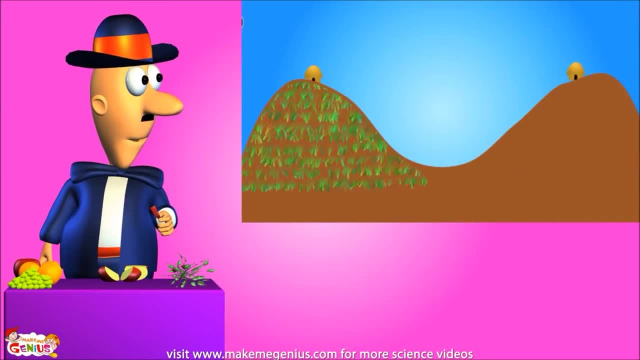 soil erosion. Look at this: On one side there are plants and on the other side it is plain land. When rain comes, plants hold the soil, so it isn't eroded on the left-hand side, On the right-hand side, there are no plants or trees, so the land is getting eroded. So we see, plants are very, very. 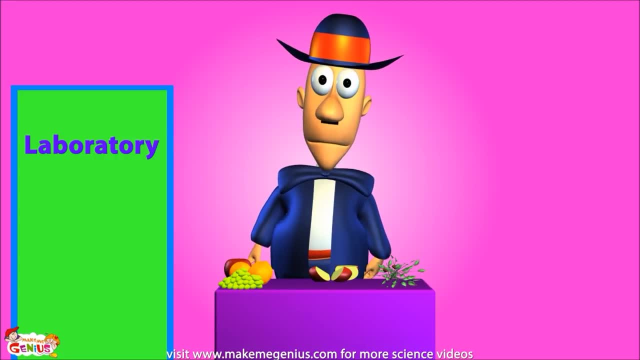 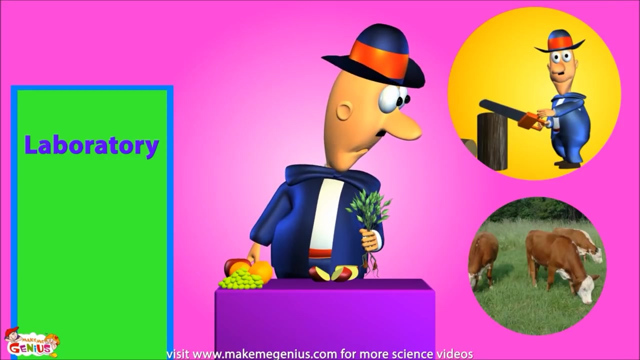 important in preventing soil erosion. so you see, plants are very important. they not only give us food, clothes and many other things, but they also save our soil from being eroded. but we humans are cutting down trees without planting new ones. we're putting more animals to graze in small areas. so the protective layer, 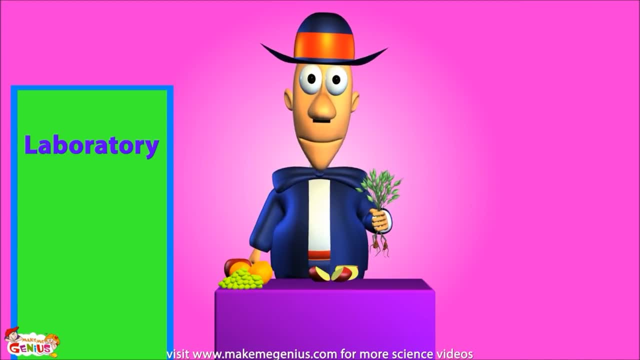 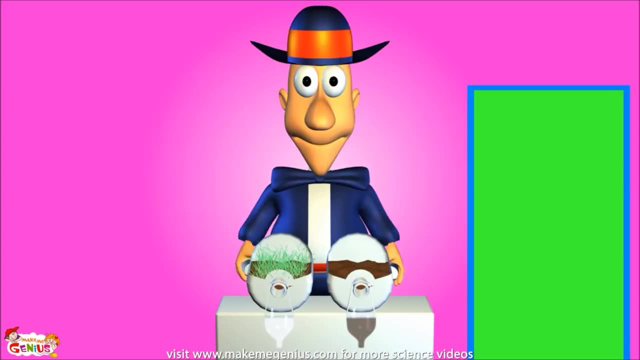 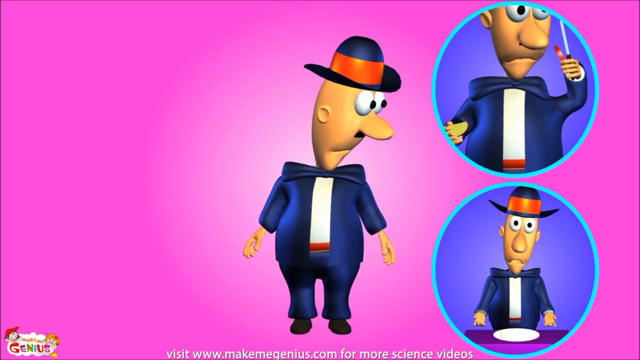 of the earth is decreasing. let's go to the laboratory and see an experiment on how plants help in decreasing soil erosion. so let's put water in both of these. so we saw today that plants and trees are very important for us. if we don't save them, then more soil erosion will occur and the area for plant growth 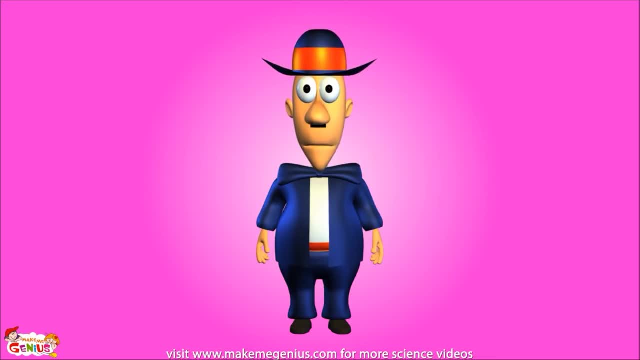 will become smaller and smaller. I hope everybody understands that we need to plant more trees and should avoid cutting them down. otherwise there won't be any soil left for growing food. here's an interesting question for you. did you know that natural erosion is good for the earth? ha ha, confused. check out the 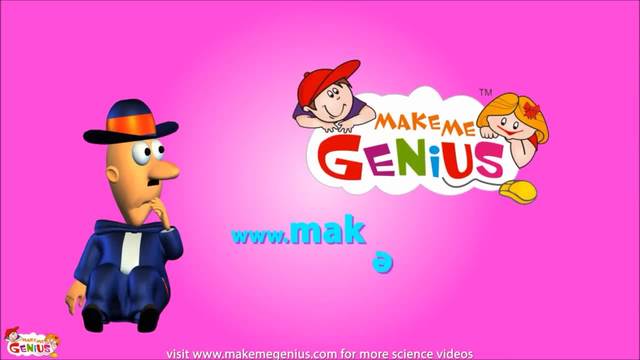 video if you want to learn more about how plants help in decreasing soil erosion, on weathering and erosion on wwwmakemegeniuscom to understand how erosion shapes our world.